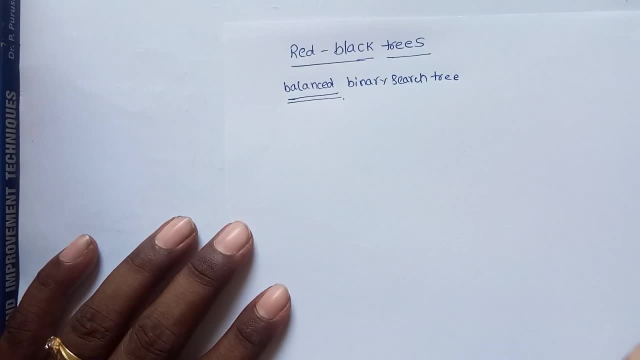 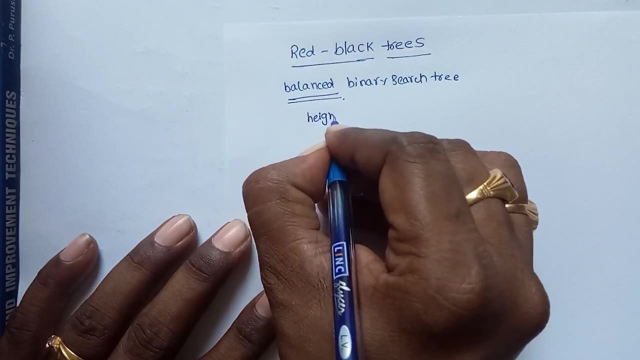 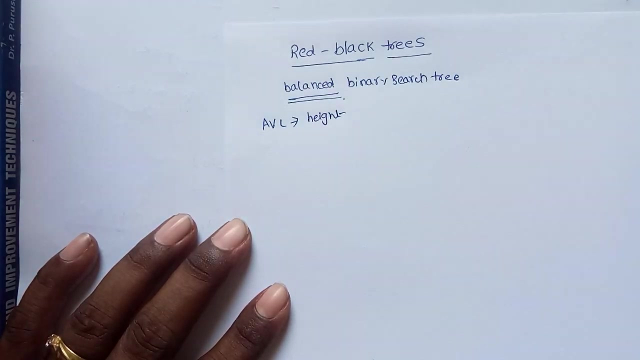 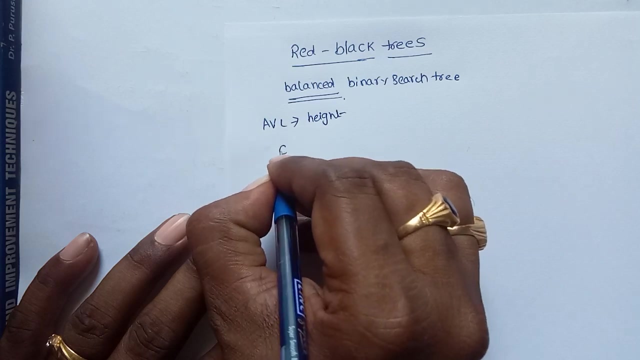 Now let us consider how the balancing occurs in red block tree. Suppose, consider an avial tree. In avial tree the balancing occurs based on height. In avial tree the balancing factor occurs based on height, That is, height of left sub tree minus height of right sub tree. is minus 1,, 0 or plus 1.. In red block trees the balancing occurs is every node is colored with red block tree. 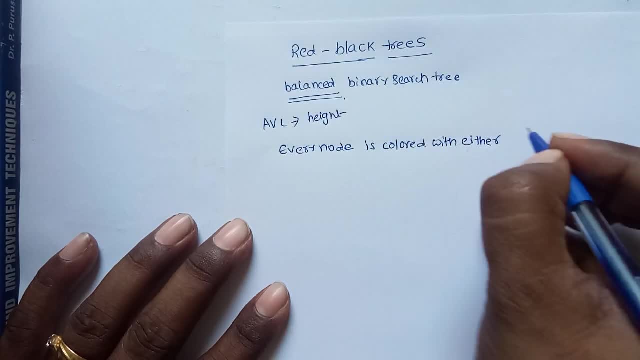 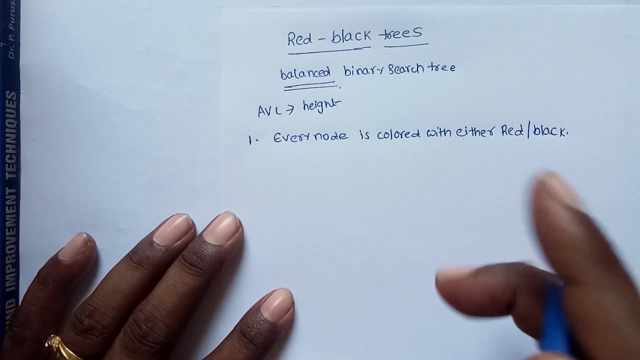 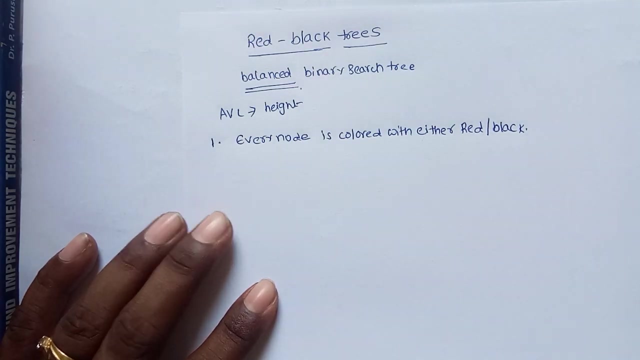 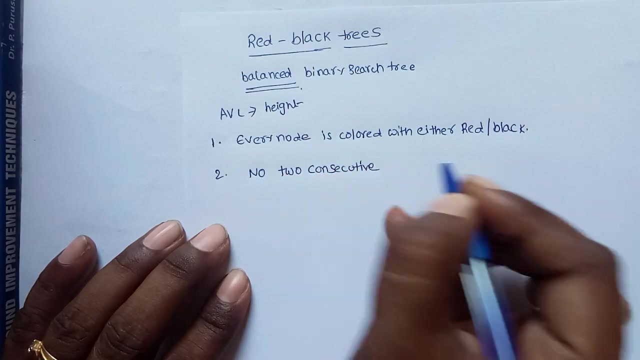 Every node is colored with either red or black, That is, the properties to make the tree as a red block tree are first property: Every node is colored with either red node or black, Either red color or black color. And another property: no two consecutive red nodes. 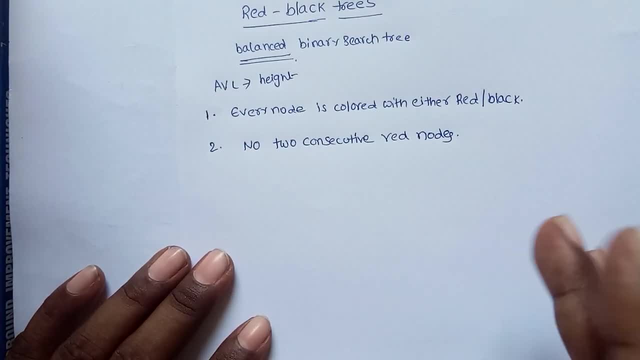 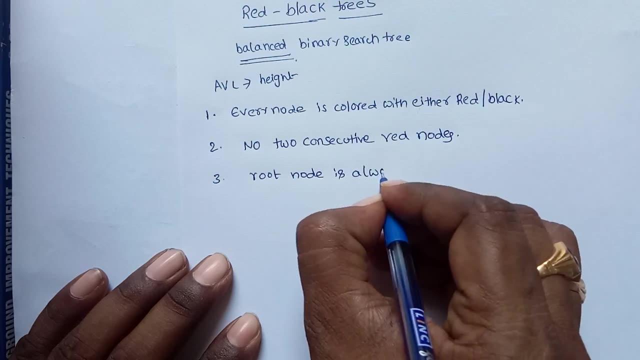 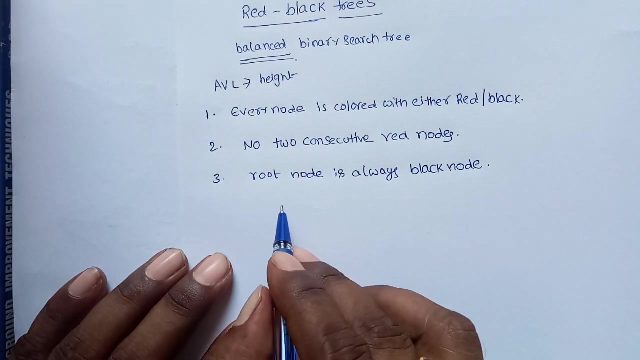 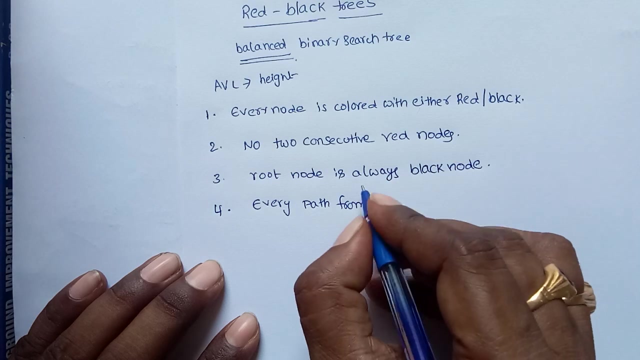 That is, two consecutive red nodes. No, two consecutive red nodes are not allowed. The root node is always black node. So the root node is always black node. No two consecutive red nodes. end, End every path, Every path from, Every path from. 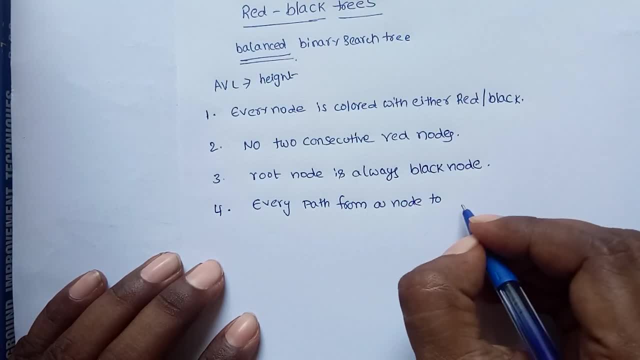 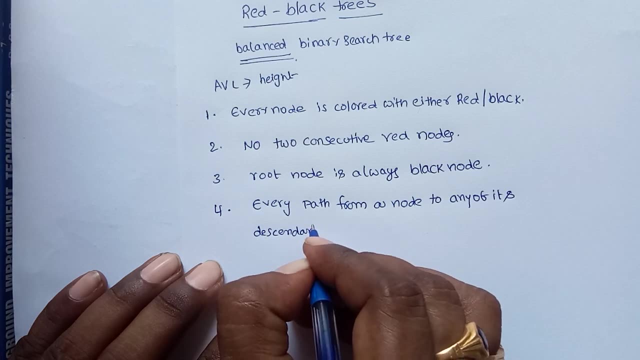 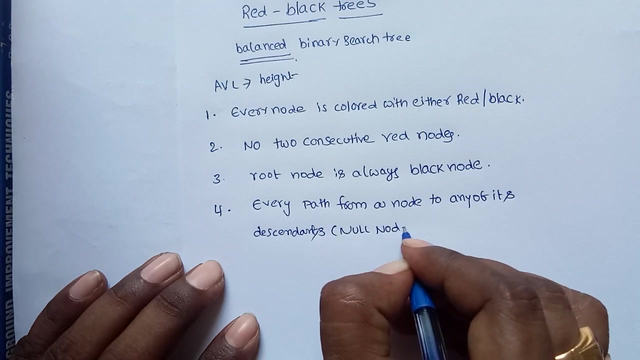 A node to Every path from a node to Any of its descendants, From a node to any of descendants Generally. here descendants means up to null node. Here leaf nodes are called null nodes. in this, For every node we have made some leaf nodes. 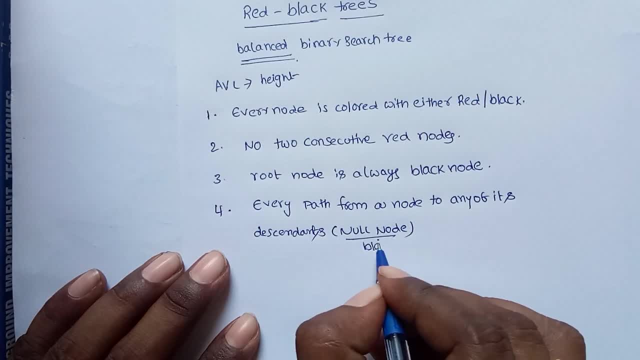 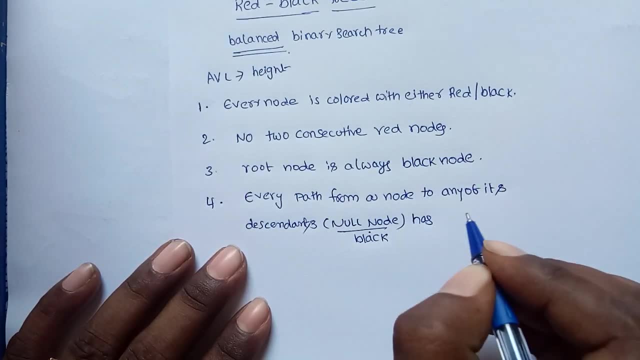 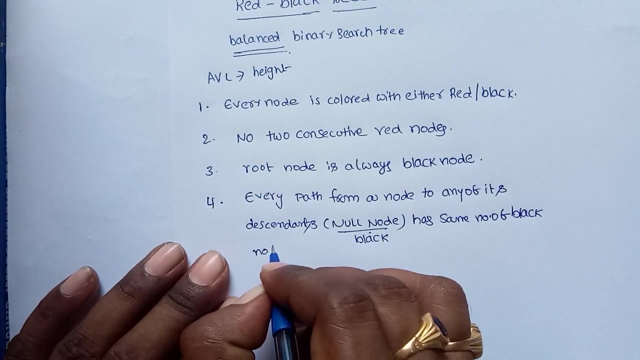 The leaf nodes are called null nodes And all the null nodes are in black color. Remember, all null nodes, Or external nodes, are in black color. Has Same number of black nodes. Have Same number of black nodes. Suppose in the tree if you are considering one node. 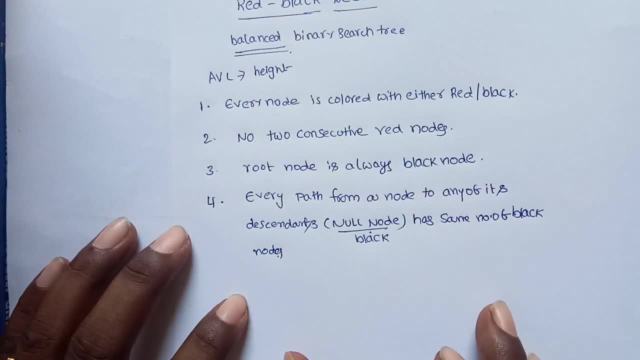 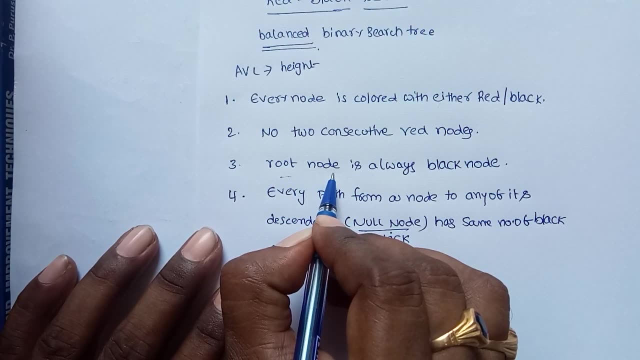 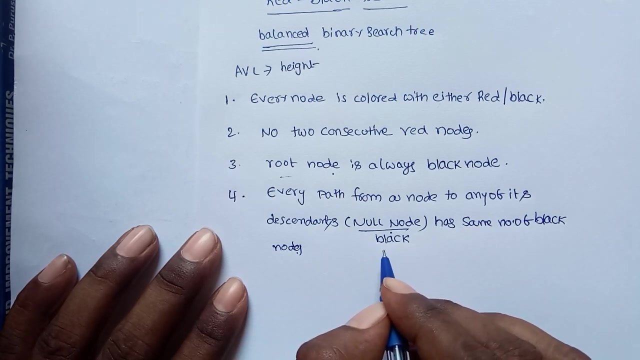 From that node to any of its descendants Contain the same number of black nodes, Same number of black nodes. Generally this is called root property. Root property means the root is always black And all external nodes, all external nodes, that is, leaf nodes, are black color. this is called external property and 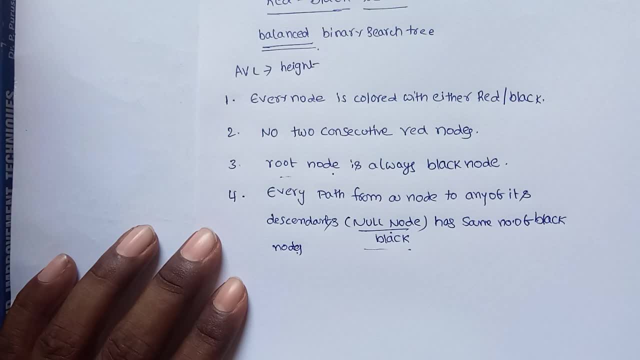 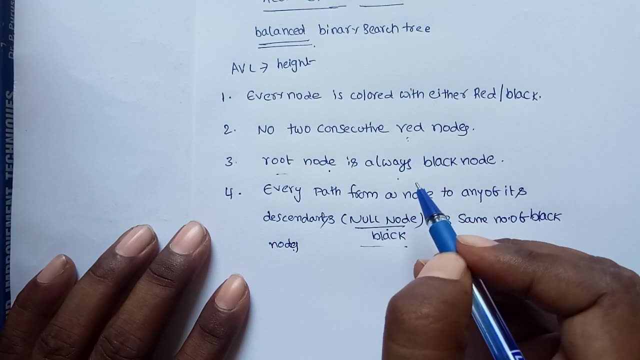 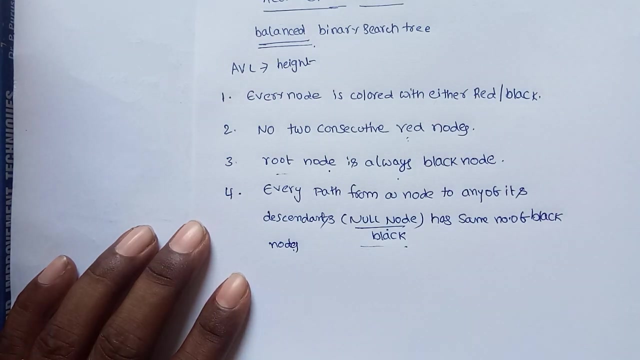 the children that is node to consecutive red nodes are allowed. that means the children of a red node is either a black node or children of a black node is either a black node. okay, and depth property means all the leaves are at the same level. all the leaves have the same level. 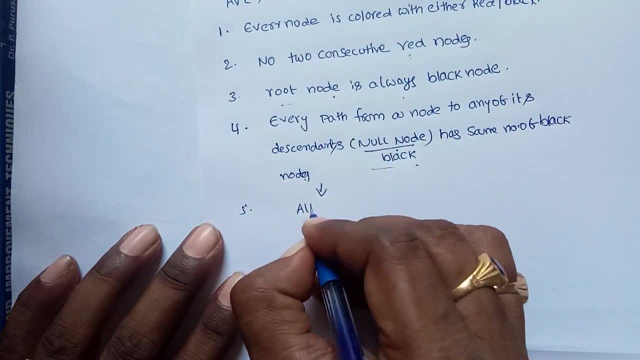 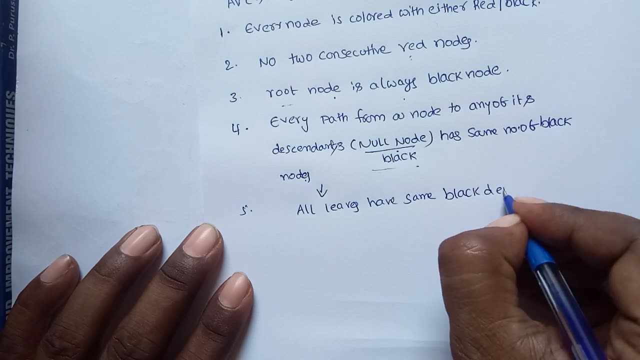 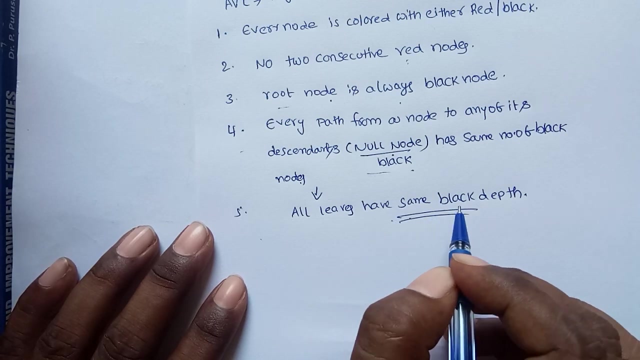 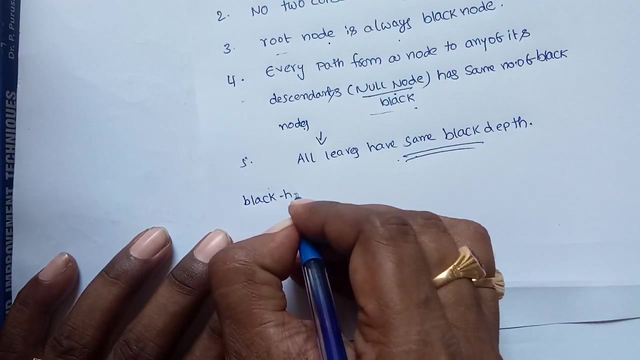 same level means addition to this point: all leaves have same black depth, remember four and five are same in simple notation. fifth one is: all the leaves have same block depth, same block depth. now I will go to one more point: block height. this is the very, very important factor. 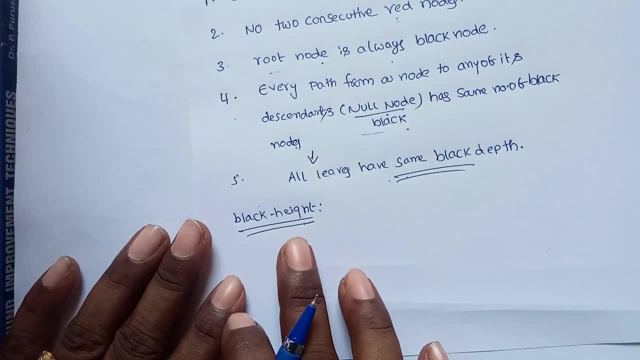 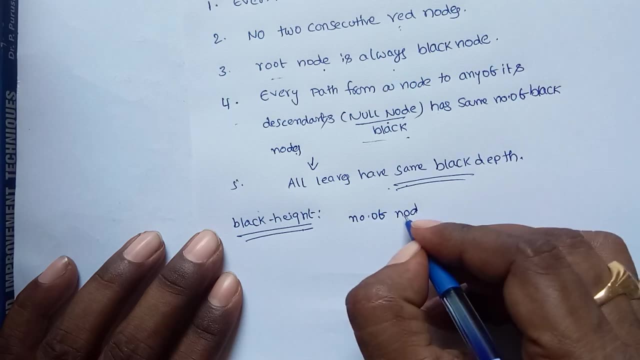 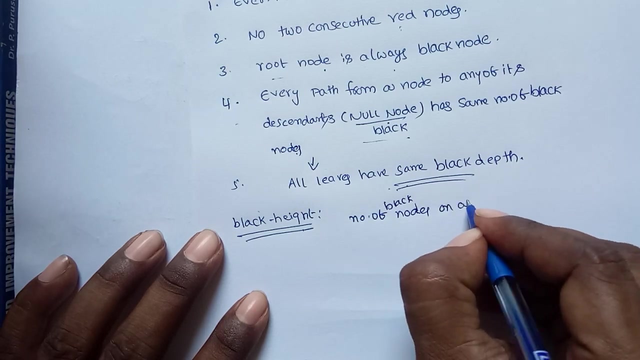 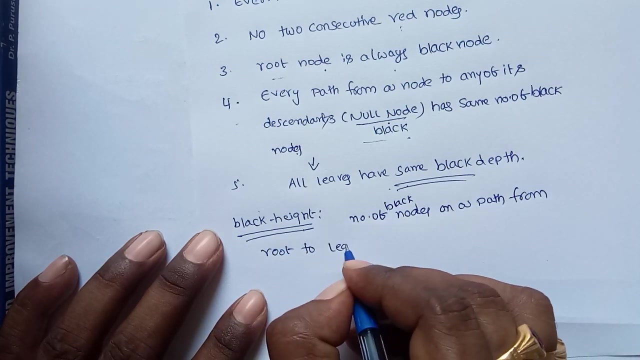 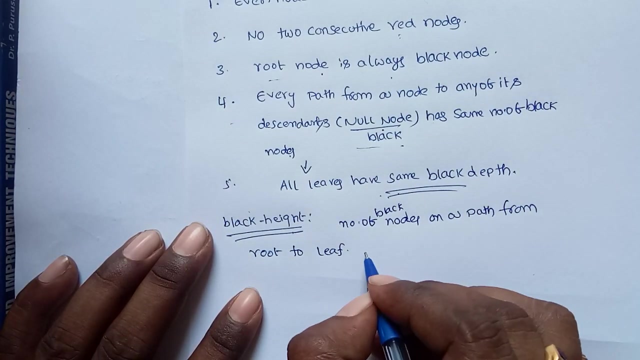 block height: black height. height of a red block tree is block. height of a red black tree is the number of black nodes. black height means the number of block nodes on a path. number of block nodes on a path from root to leaf. the number of block nodes on a path from root to leaf. here leaf nodes also counted as. 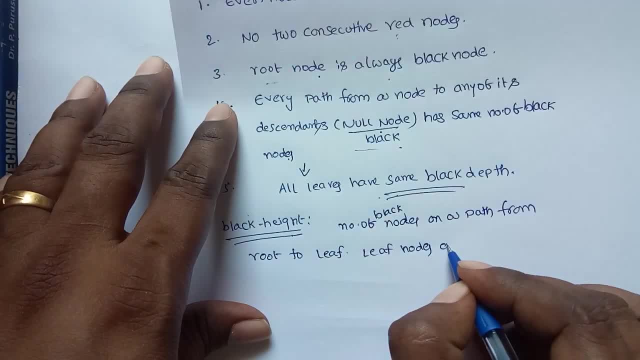 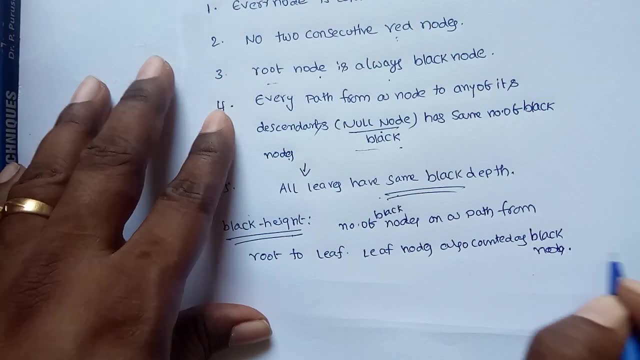 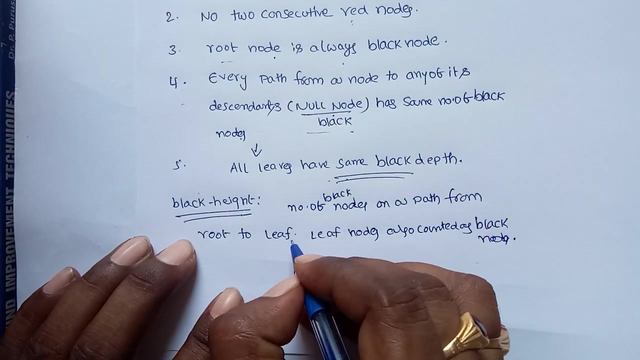 black nodes. remember leaf nodes are external nodes. leaf nodes also counted as block nodes, also called as block nodes. this is the black height. black height is the number of block nodes on a path from root to leaf. this is the black height. for example, h is the height of a red block. 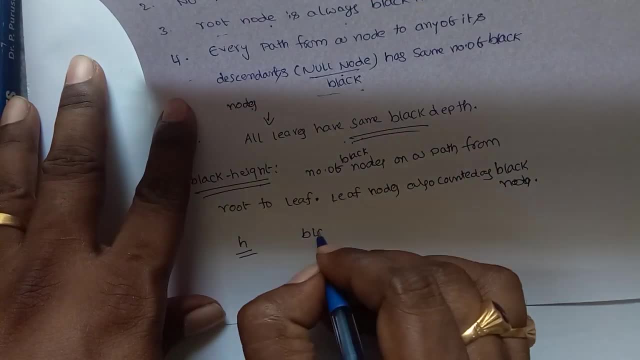 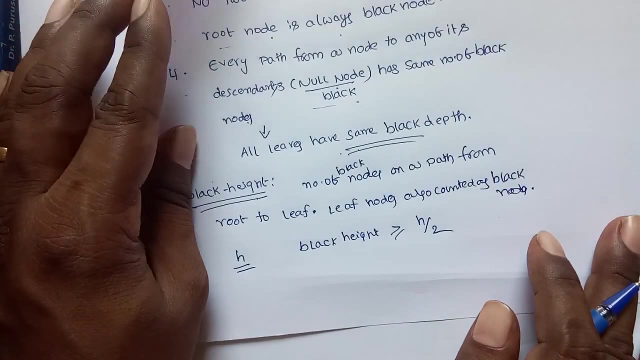 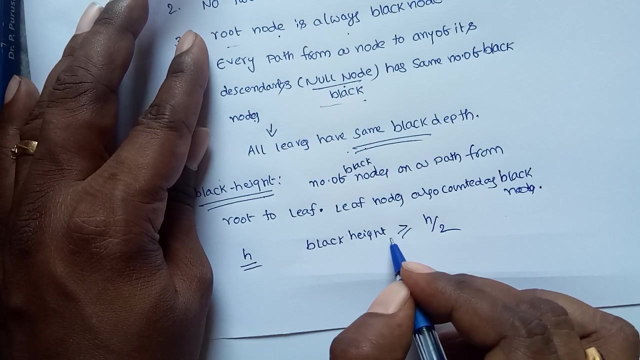 tree. if h is the height of a red block tree, then remember the block height is greater than or equal to h by 2. the block height is greater than or equal to h by 2 because there is a chance, for half of the nodes are red nodes and compulsory node 2 consecutive to red node means compulsory. 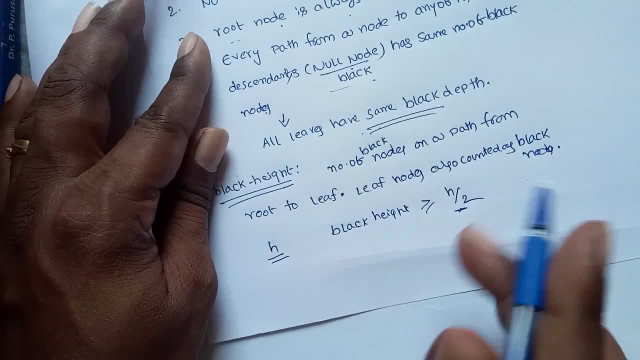 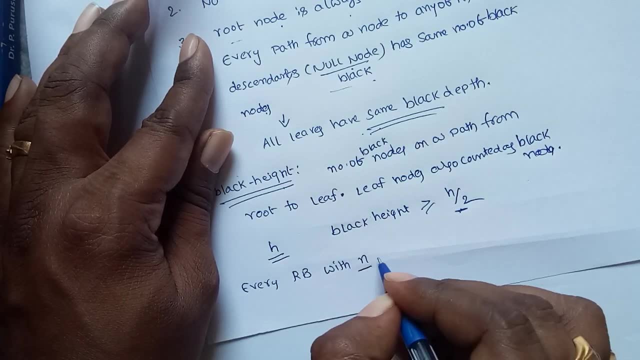 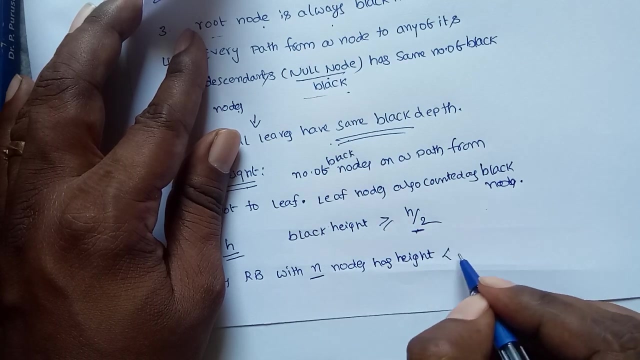 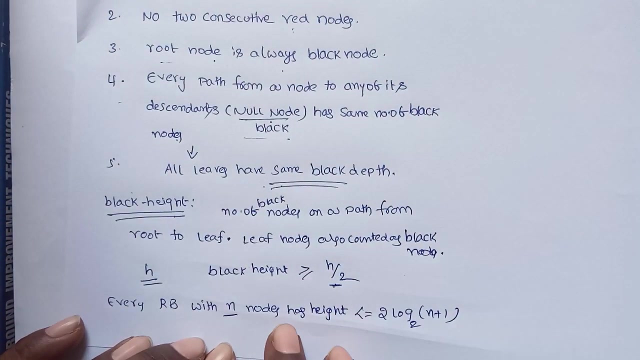 more than one block node height is greater than h by 2 and one more. every red block tree. every red block tree with n nodes. a red block tree with n nodes has height less than or equal to 2 into log 2 n plus 1. every red block tree of height. 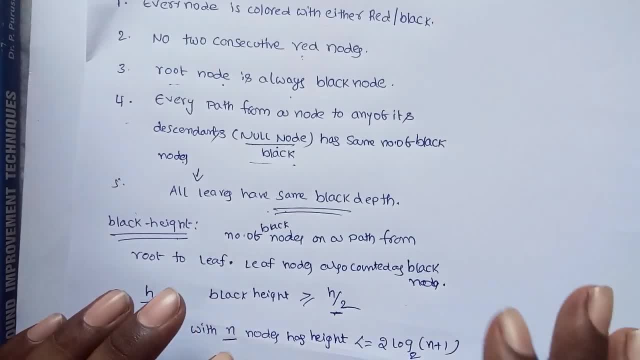 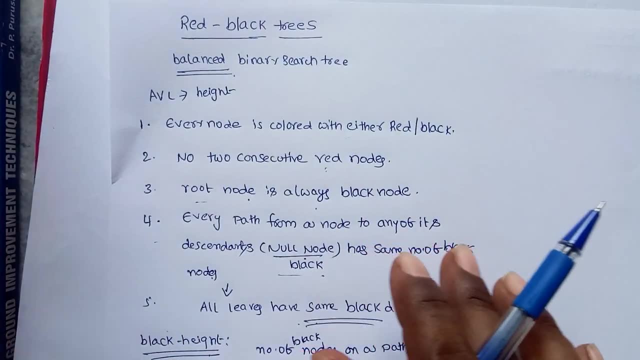 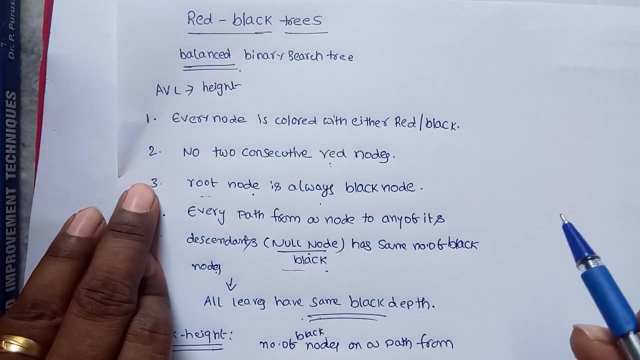 n. this is the formula. okay, so we already know binary search tree. and after binary search tree we discussed avl tree. avl tree is also a balanced binary search tree. then what is the need for right block trees? suppose in avl trees the insertion or deletion operation takes more number of rotations? 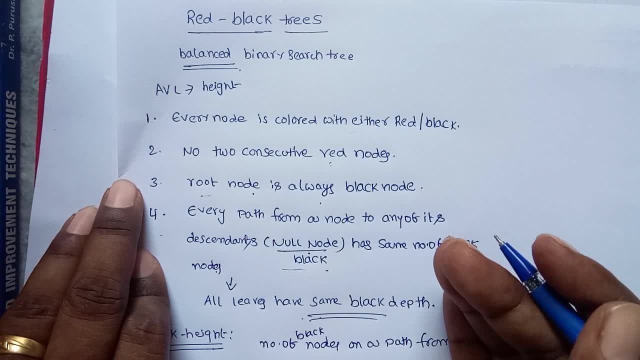 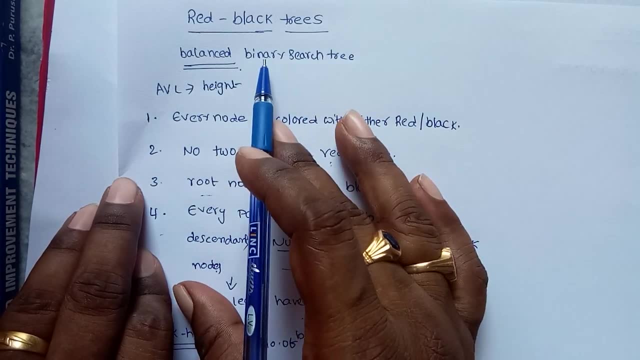 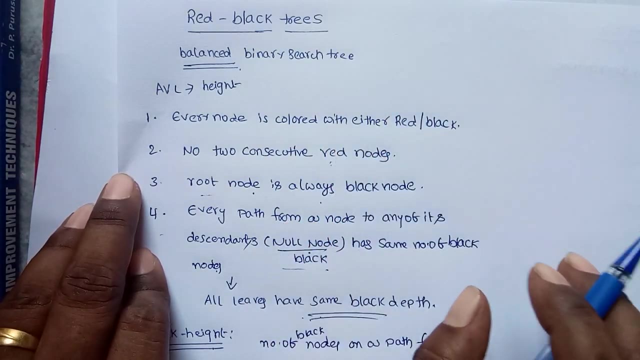 if you want to perform many number of insertions and deletions, simply avl tree is not preferable. in this case, we are moving to red block trees. in this case, we are moving to red block trees. why? because in red block trees the number of rotations are less compared to avl trees. okay, and 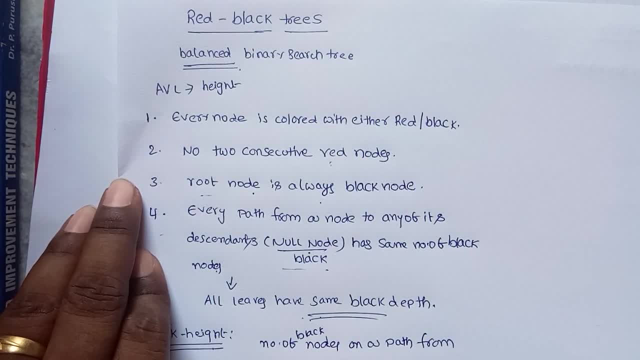 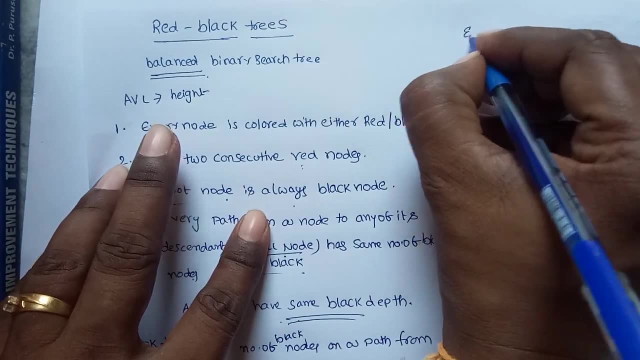 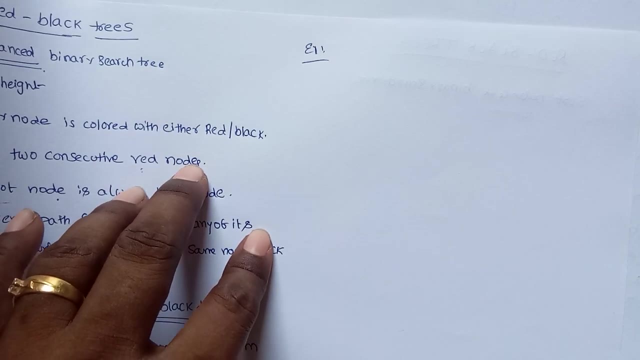 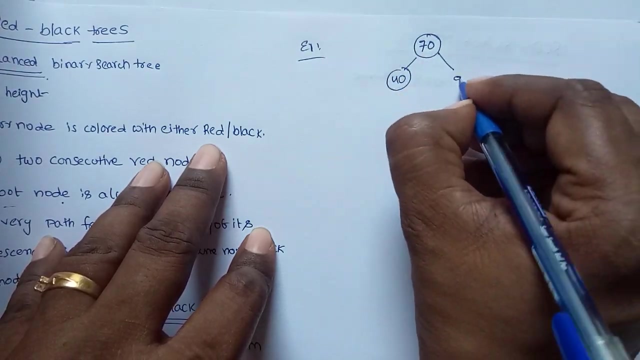 if you are to perform search operation, if you want to perform search operation, avl tree is preferable, tree is preferable. okay, now consider an example. consider an example tree that is to represent an avial tree and check each and everything: 70, 40, suppose some example: 30. 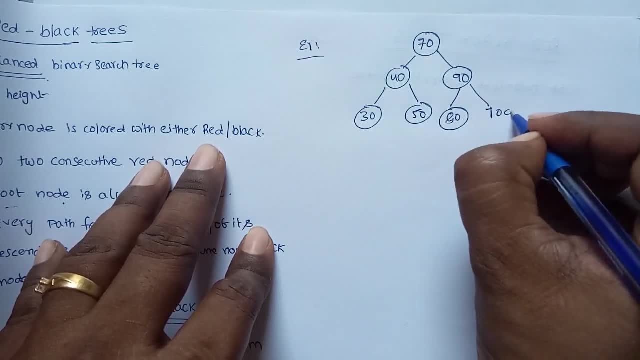 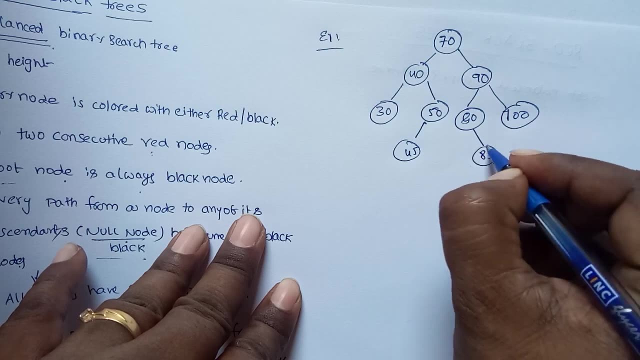 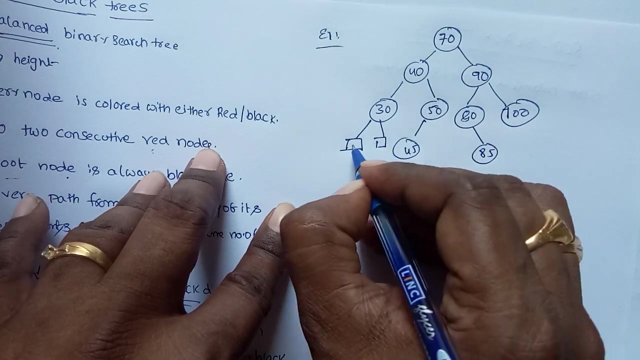 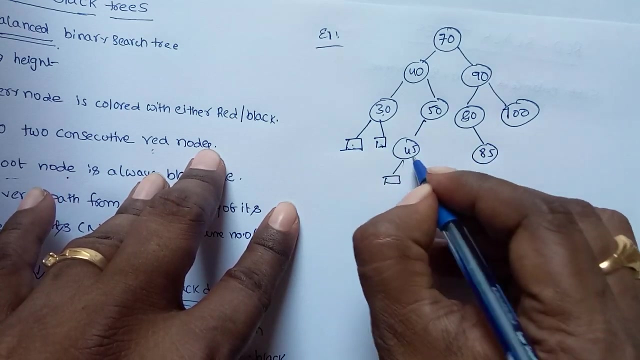 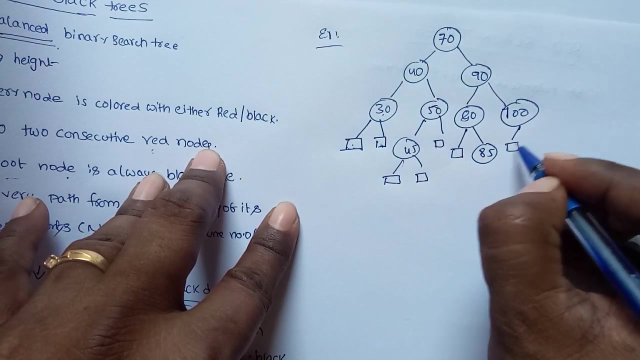 50, 80, 100, for example. these are the given nodes. and remember, all external nodes are. these are the leaf nodes. now, these are the leaf nodes. this is not the leaf node. these are the leaf nodes. all external nodes are colored with block, also called as null nodes. suppose the value is. 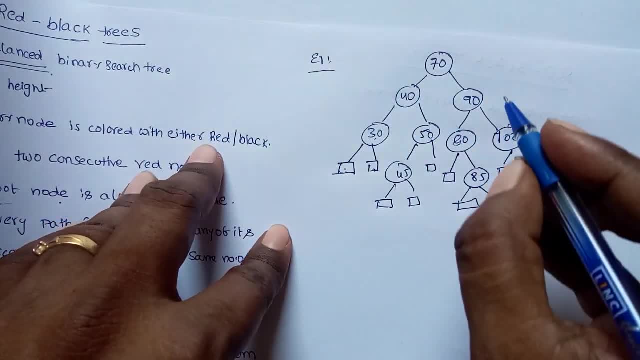 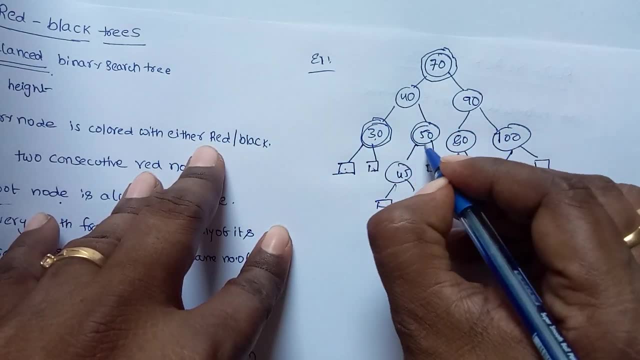 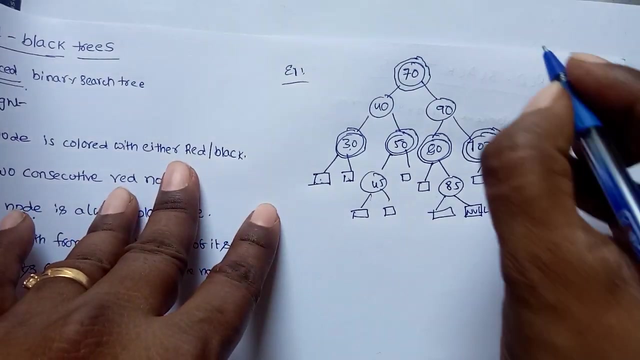 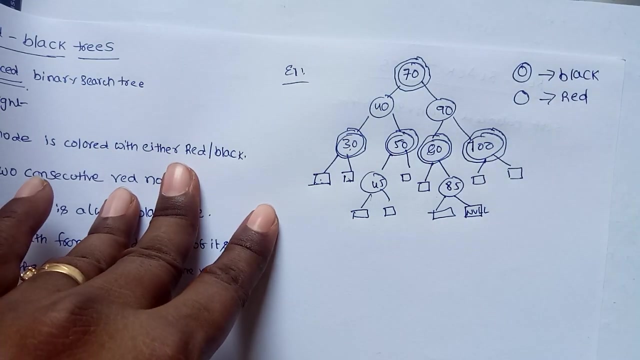 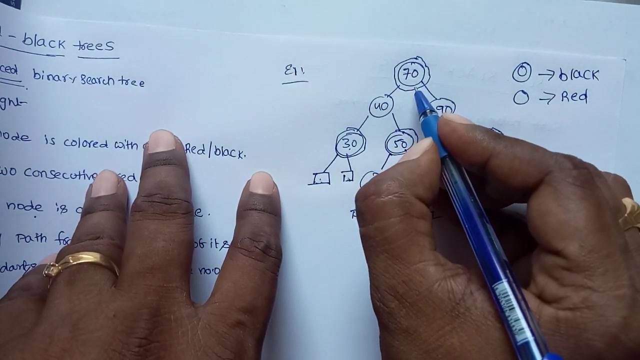 null node. the value is known. the root node is always block node. suppose given tree. suppose for simplification: double circle represents a black color, single circle represents red color, double circle represents black color, single circle represents red color. see this one. check the properties: the root node is always block node and first point is it satisfies the binary history property. 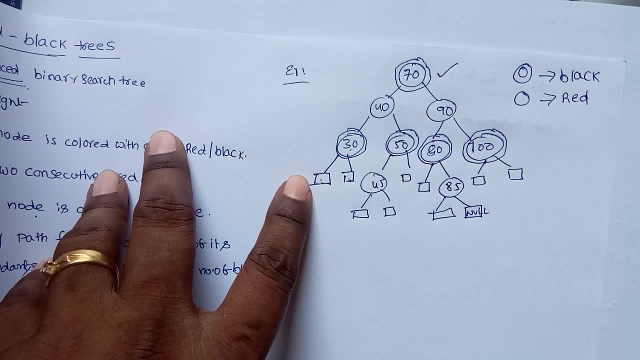 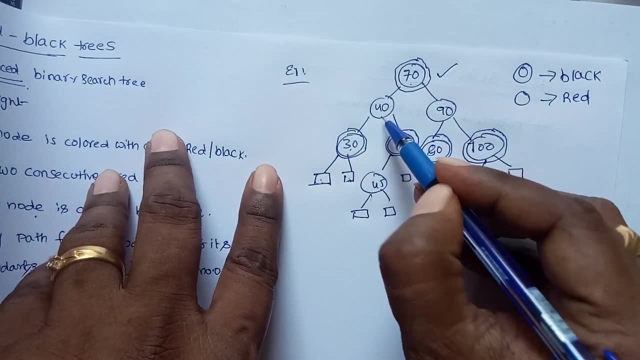 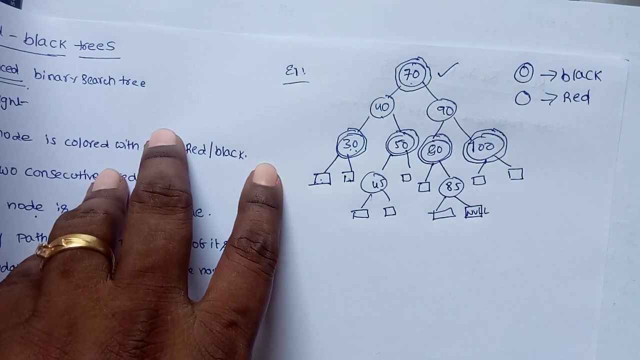 the root node. 70 is a block color satisfied. then the next one is no two consecutive red nodes. see this one: 70 is a block, 40 is red, 30 is the right block, so see any any level. no two consecutive red nodes are present, so it satisfies that property also. that means the children of a red node are. 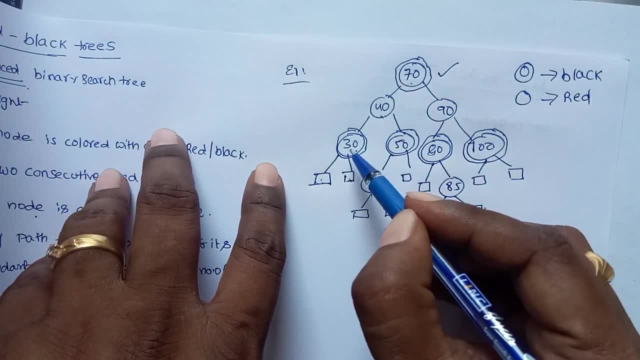 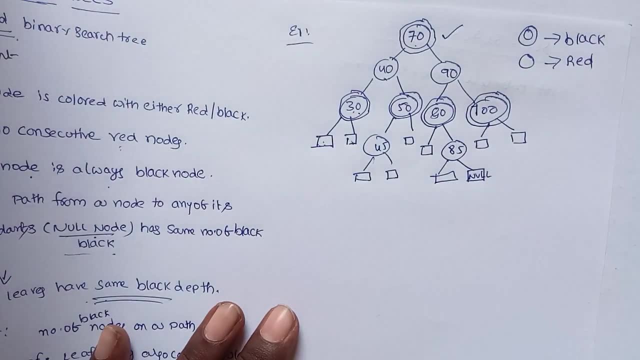 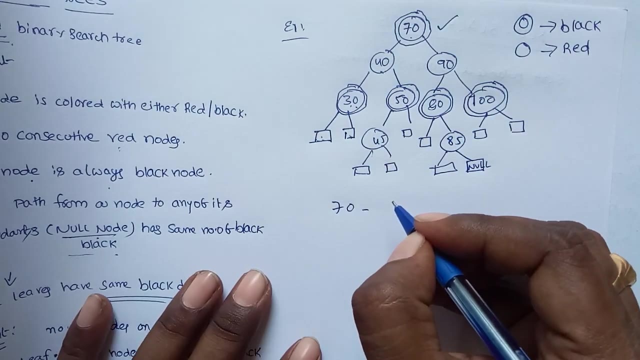 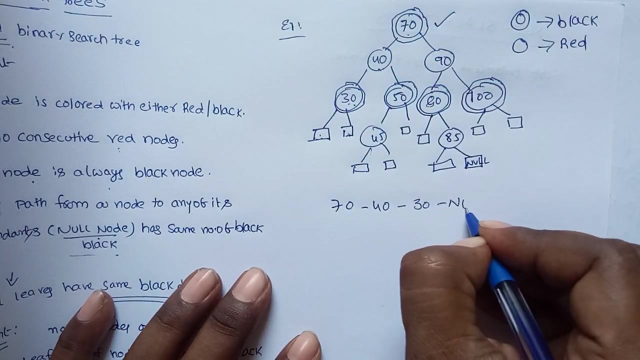 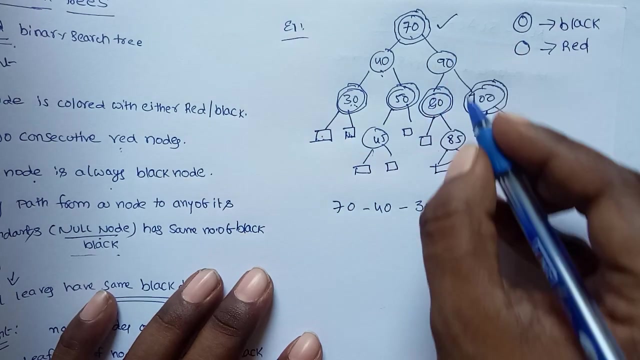 even redester red and then the checkbox and end as red locked. apologize, this one is for black block to get appreciated. now let's see how to calculate. if this set is not implement snow or block no two consecutive means, the children of red nodes, or compulsory 40, 40 to 30, 30 to some null node, suppose some another path: 70, 70 to 90, 90 to some 80. 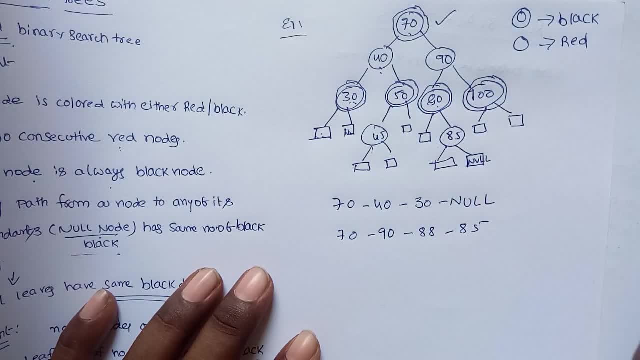 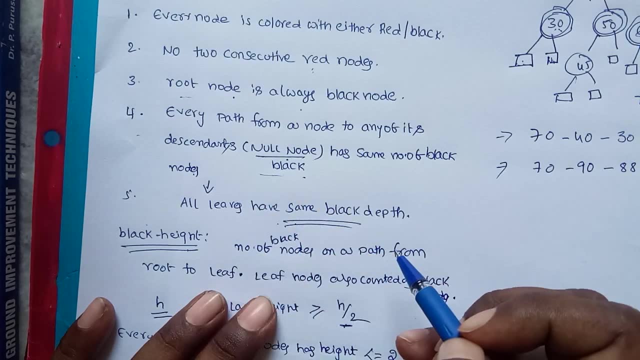 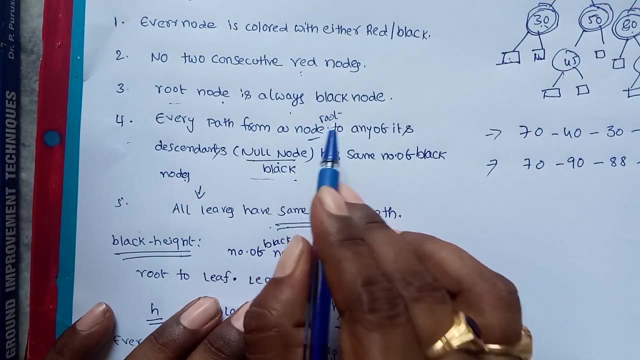 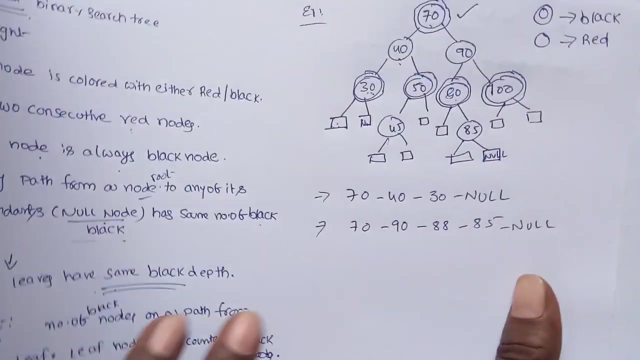 80 to some 85, 85 to null. see this one. here the property is the number of block nodes. every path from the node- here from the node means, suppose, consider the root node, the path from root to any of its descendants have same number of block nodes. have same number of block nodes. see the path. 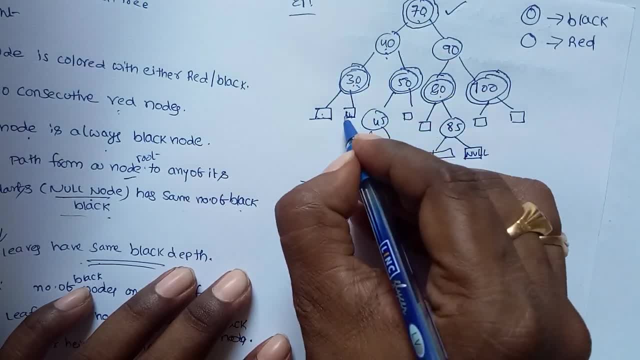 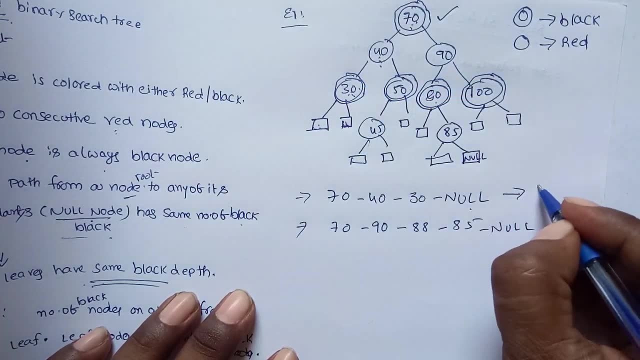 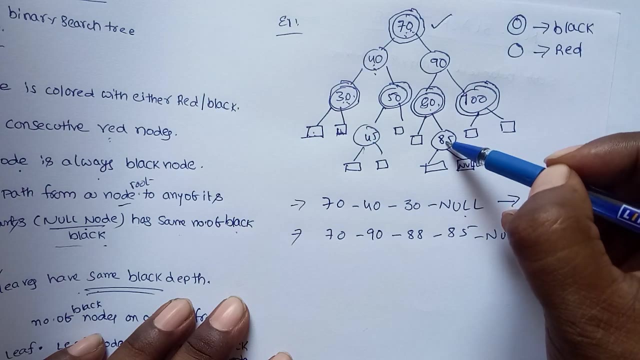 70, 40, 30. i am rooting the null node. this is one path. how many number of block nodes? one, two and including null three. it contains three block nodes, suppose. consider this path: 70, 90, 80, 85 and null. 70 is one, 80 is another, null is three again. 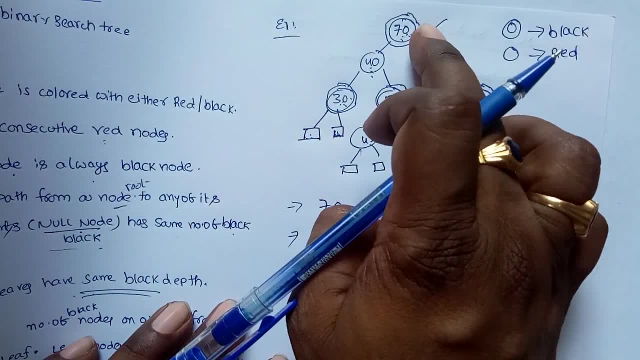 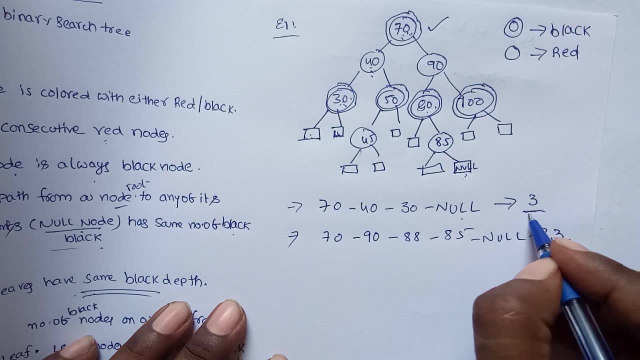 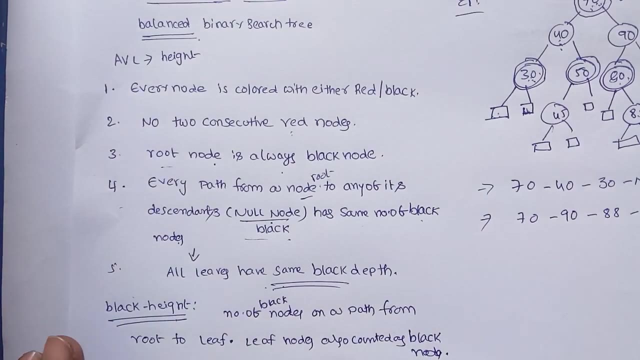 three block nodes, okay, every path from root. two on any of its descendants, that is, from root to null node on any path. the number of block nodes must be same. the number of block nodes must be same. this is the insertion. sorry, this is the introduction to red block trees, the only main. 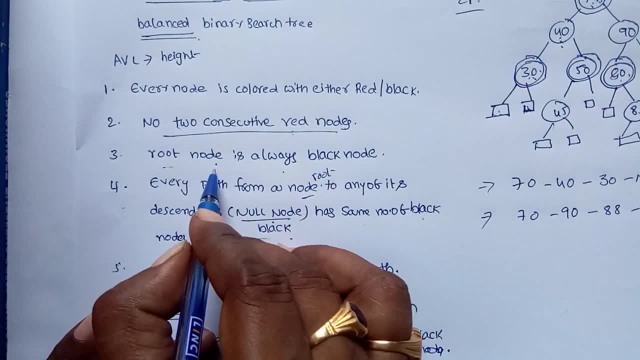 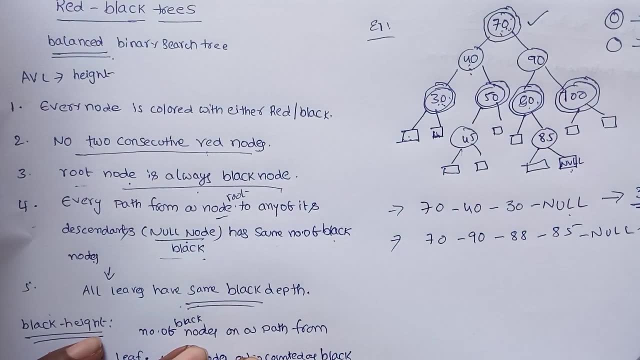 properties is node to consecutive red nodes. the root node is always black node and every path from the root node to any of its leaf node contains the same number of block nodes. in the next session we will discuss insertion. thank you.